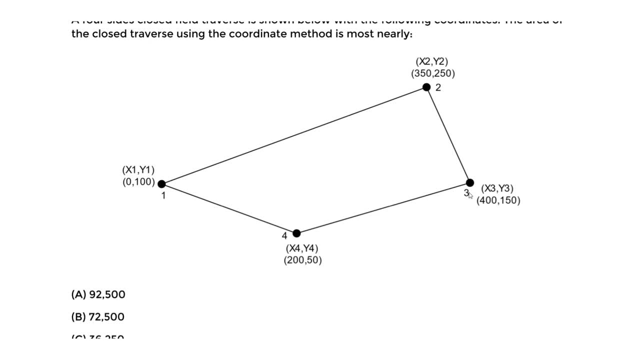 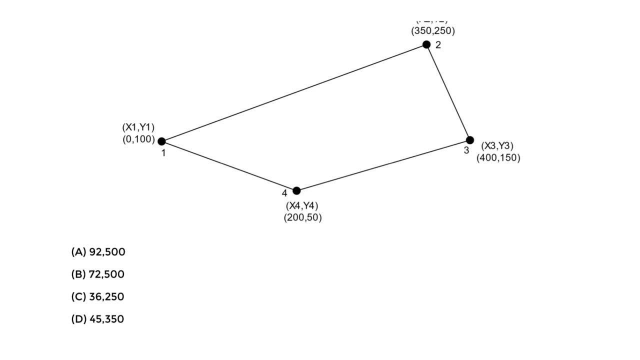 Because in the handbook that equation can look messy and quite confusing. So the way we will solve this question is first denoting two rows. We know we start at x1, go to x2, go to x3, go to x4, then end back at x1. We have to close that traverse right, Or else we do not have an area, a closed area. So we have to start at x1 and end at x1.. So we will draw this as the first row. 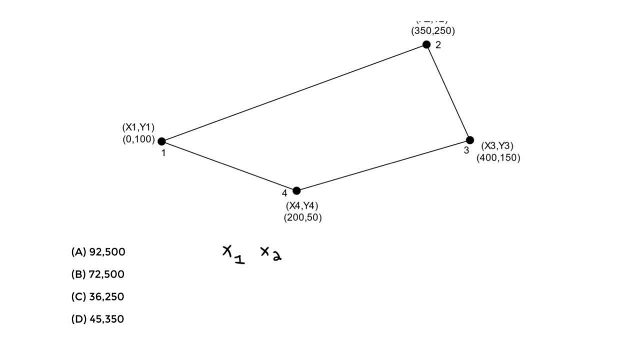 So we know this will be x1, x2, x3, x4, then we end back at x1, right, We start at x1 and we close at x1.. It's a closed traverse, So that will be the top row. So I'm going to denote two rows: The top row and the bottom row. The bottom row is going to be for the y values, So we just do y1, y2, y3, y4, then we end at y1.. 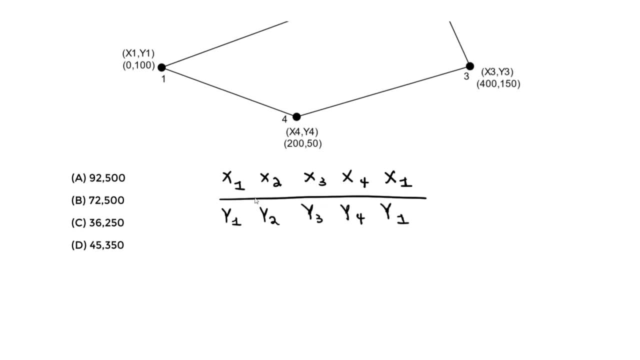 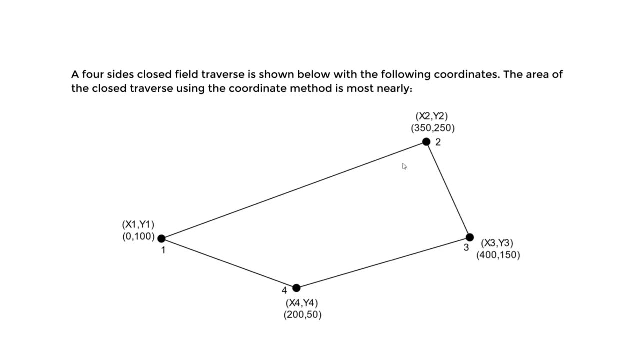 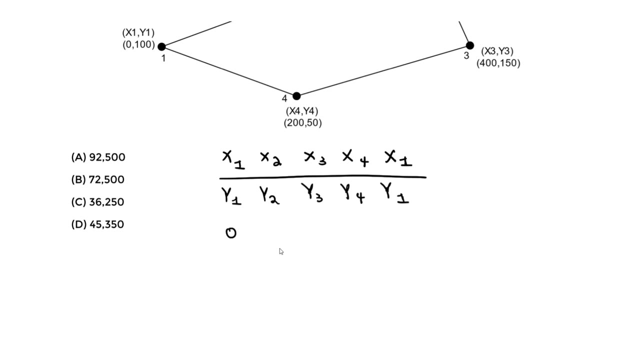 So we have these two rows. So now let's fill out the appropriate values. So we're doing this to use a certain method and to visually solve using the coordinate method. So we have the top row, bottom row, and let's put the values. So x1 is 0.. We know x2 is 350, x3 is 400,, x4 is 200, and x1 again is 0. So we plug in the 350 for x2.. 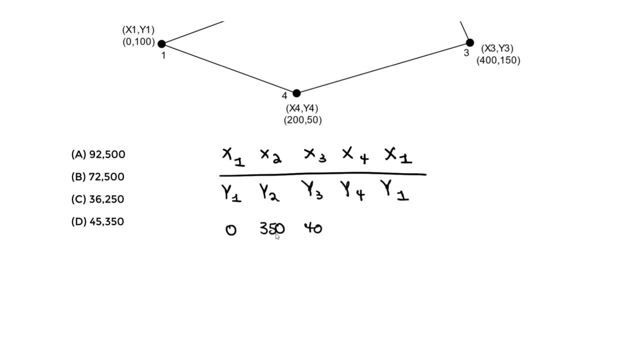 We plug in x3, which is going to be the 400.. X4 is going to be this value, so 200. Then we end at 0. Then the bottom one is going to be y1, so it's 100.. Y2 is going to be 250.. Y3 is going to be 150. And y4 is going to be 50. Then we end back at y1.. Again, it's 100.. 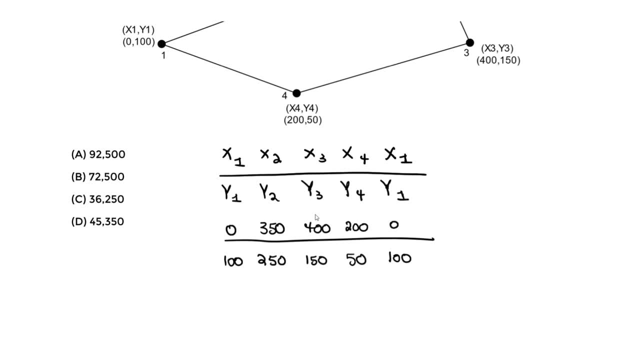 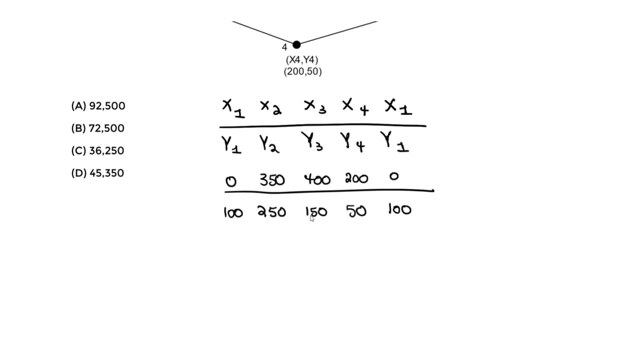 So we have the top row and the bottom row. So this is going to be the first step you do when we're looking at these coordinate method questions for a survey. So then what I propose is something similar to the cross product. You might recall this. So what we do for these questions is essentially the following: 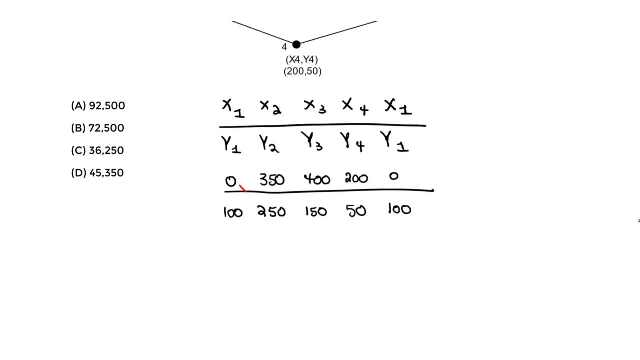 We take 0 times 250 minus 100 times 350. Then we do plus 350 times 150 minus 150. Then we do minus 250 times 400. Then we do plus 450 times 50, and you get the point here. 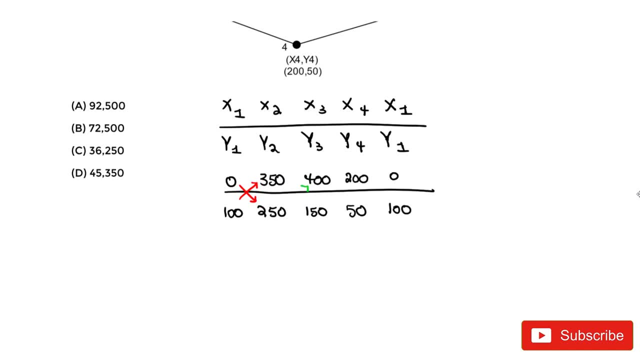 But we'll do it step by step. So let me erase this, Erase the ones in red. So we have that. So let's start with 0 times 250 minus 100 times 350.. Don't forget that minus. So I'll write this: 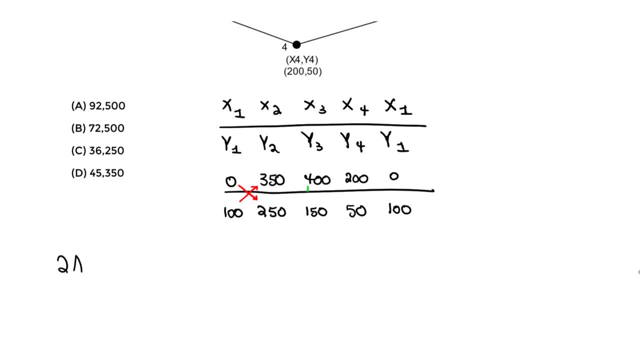 So we know the total area. It's going to be 2 times the area. That's why we divide by 2 at the end, which we will show. So we do 0 times 250 minus 100 times 350.. 100 times 350.. 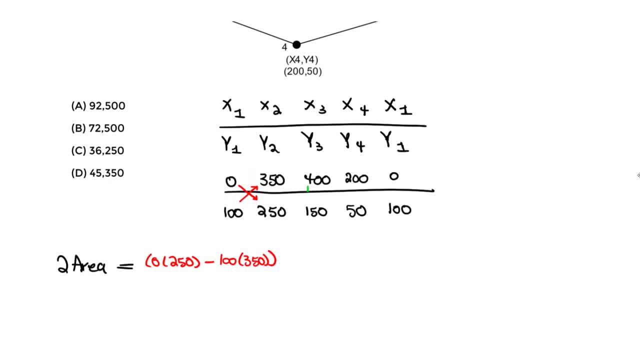 Open parentheses, close parentheses, And that's taken care of. Now we move on to the next step: 350 times 150 minus The 250 times 400.. So we do plus, Don't forget this. plus Now we do the one in green. 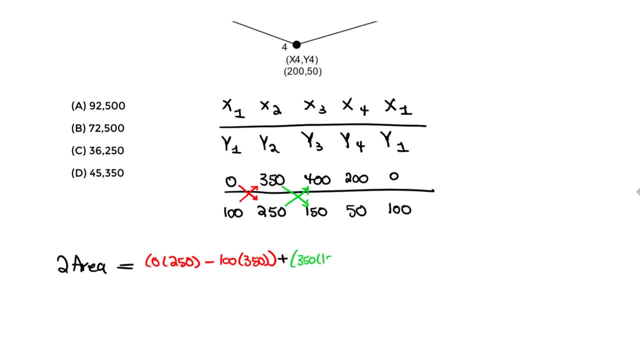 So we do 350 times the 150 minus 250 times 400.. Close parentheses. We move on to the next step. So we do this color. Let's do pink. So we do 400 times 50.. 400 times 50 minus 150 times 200. 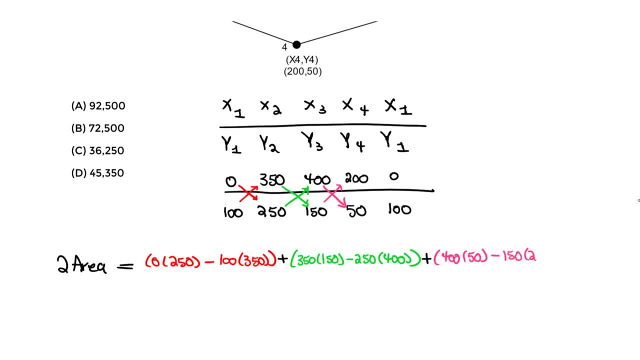 So we do 150 times 200. And close parentheses, And the very last one is going to be this one, right? So we do 200 times the 100 minus 50 times 0.. So we do plus And I'll put this down here.